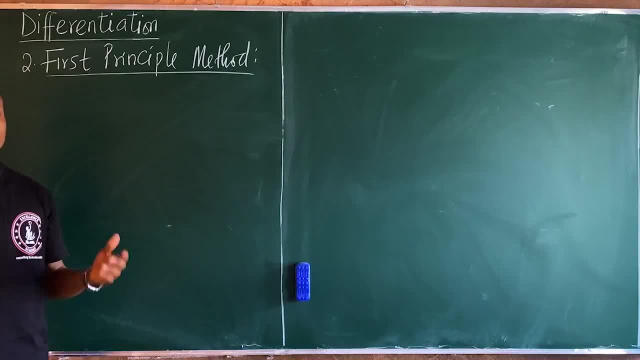 I'll just take an example and we explain together, right, All right. so example one: under first principle, let's say I have y being equal to x From the idea of general method we've done before now, I'm going to take x and I'm going to take y, and I'm going to take y and I'm going to. 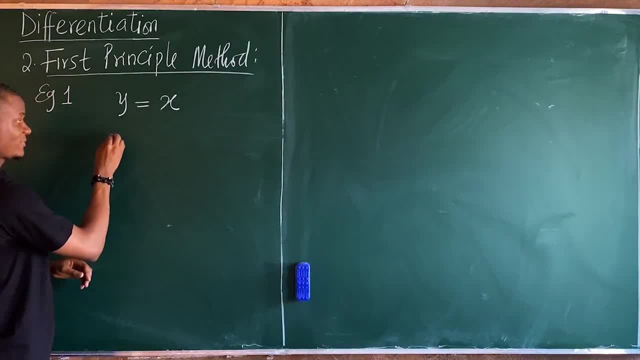 I'll have that. this will give you 1.. Here's the concept I'll have that. the y over the x is equal to, we said, multiplied by the power. The power here is 1.. So it becomes 1 times x into what's. 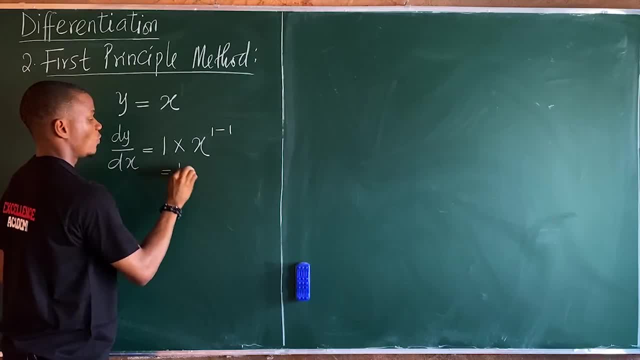 there 1 minus 1.. This is equal to 1 times x. into 1 minus 1 is 0. That's now equal to 1 times x. gives you what there? 1.. 1 times 1 is 1.. This is the general method of. 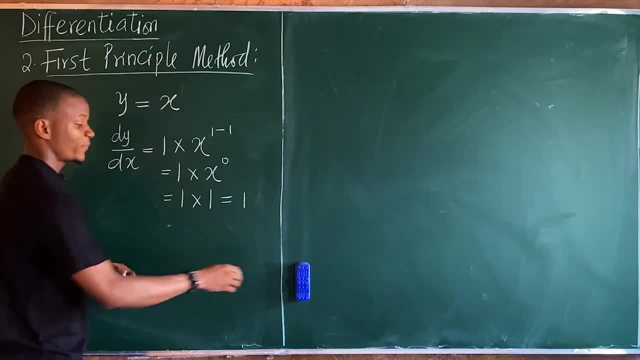 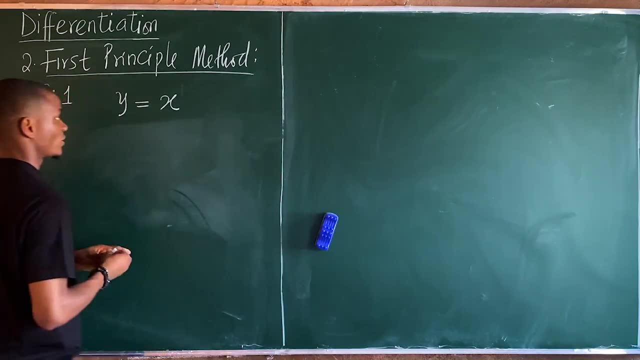 solving this question. If I'm to use first principle method, what do I do? What's the concept of first principle? Now, here's your idea, please, For first principle from this function. your first case is to add change in y to y and then add change in x to x, So I'm having y here. 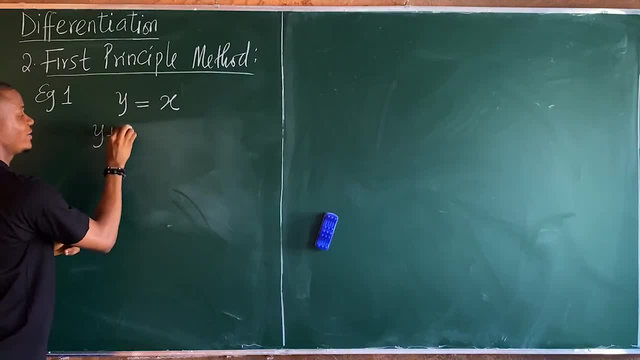 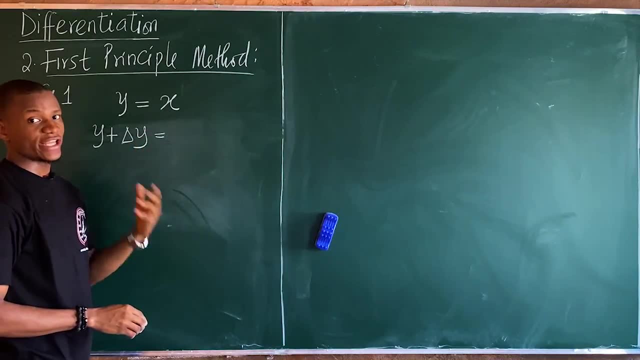 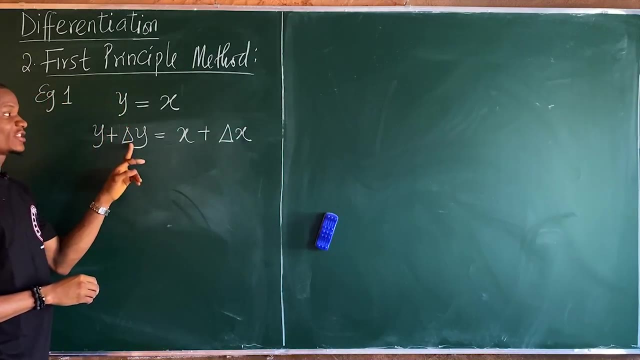 It becomes y plus. I said to y: add change in y is now equal to here x. I said for x: add change in x becomes x plus change in x. So it's simple enough to y add change in y to x: add change in x. Next up I'll move y over here, So I'll have that. 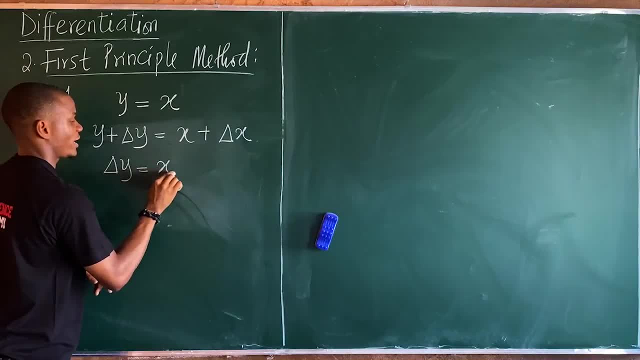 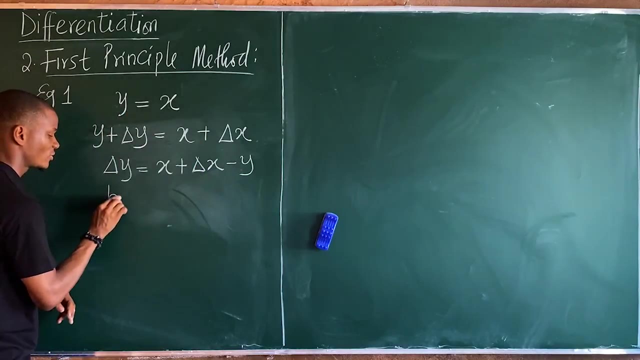 change in y is equal to x plus change in x. Here's a plus y Concept becomes what there Minus y. Next up, I'll substitute the value of x from this point here. but we just said from here that y is equal to what there X. Hence I have that change in y is equal to x plus change in x. 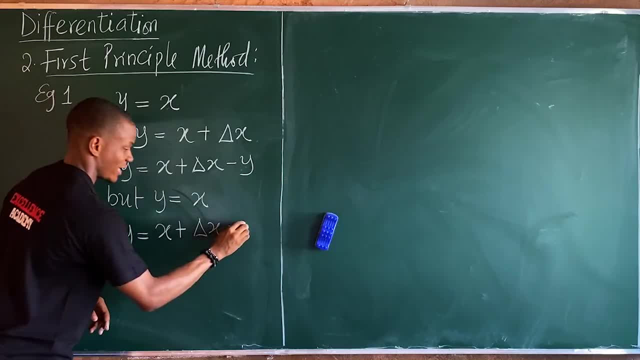 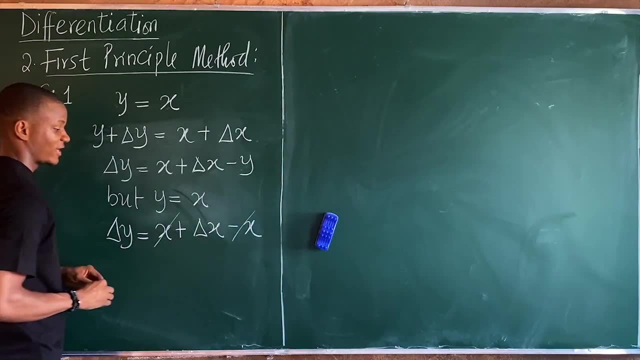 minus y. What's y? Y is x, It becomes x. From this it becomes x and minus x. So x cancels minus x. i'll have that. change in y is equal to change in x. so next up: divide true by changing. 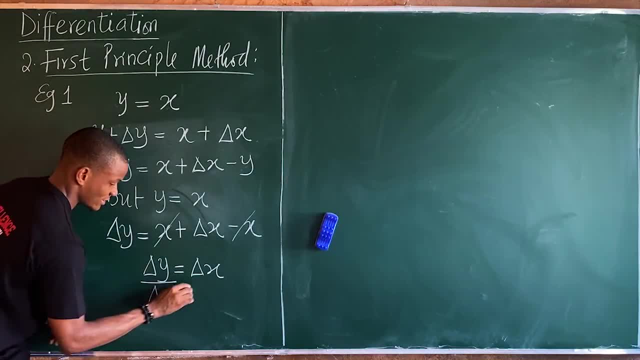 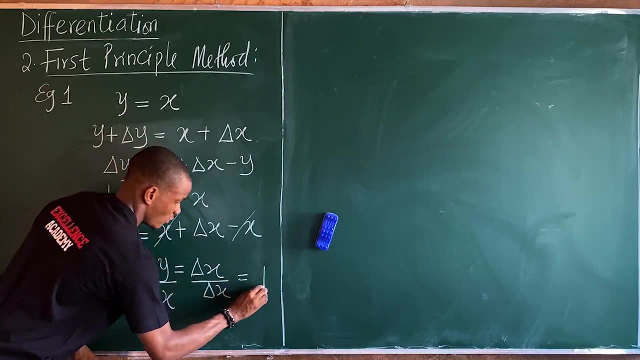 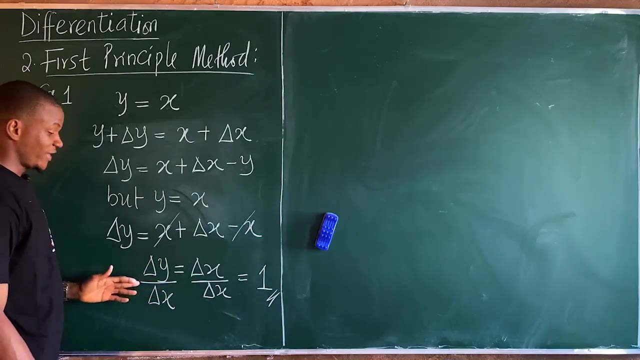 x, it becomes all over changing x, all over changing x, and this is now equal to changing x over changing x. gives you what the one? so this is the answer. remember, when i did this using general method, i had one. so, using first principle, i'm still saying one. so this is the simple concept behind first. 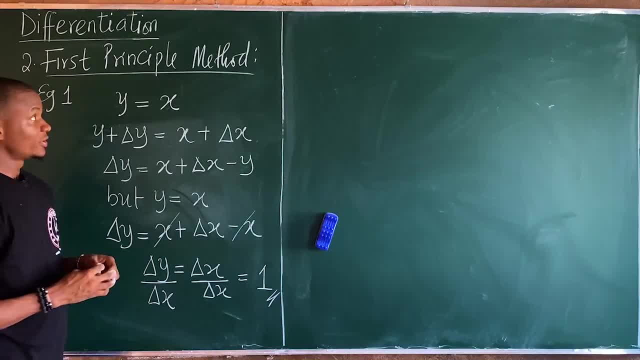 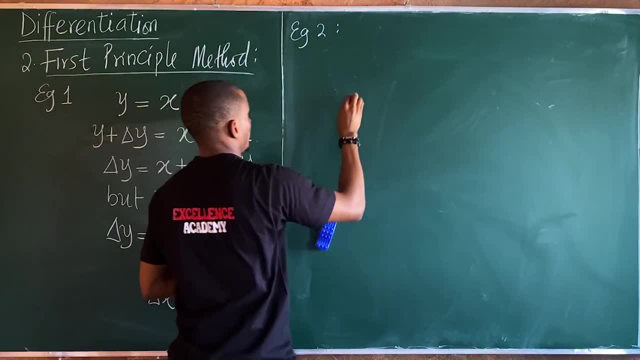 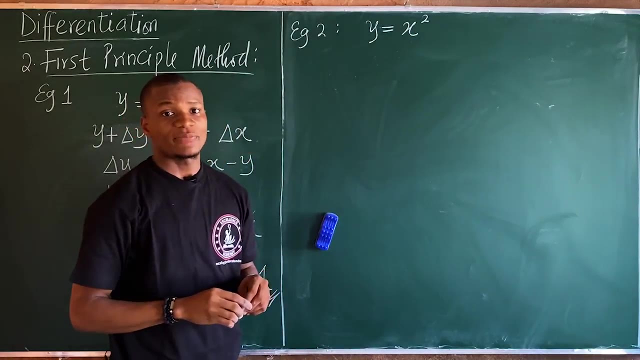 principle method of differentiation. take another example under first principle. so under first principle, let's take example two. let's say i'm giving y being equal to x square. from this, if i use general method, obviously i will have that dy over the x is equal to x over x. 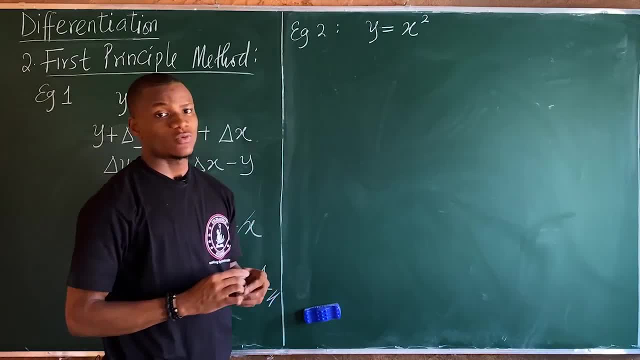 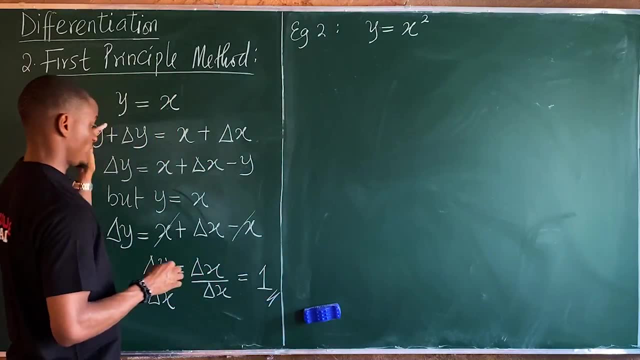 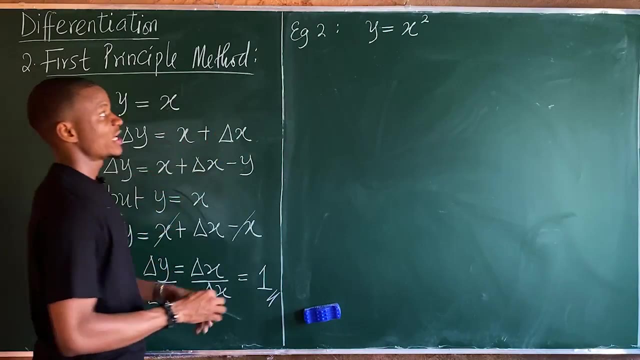 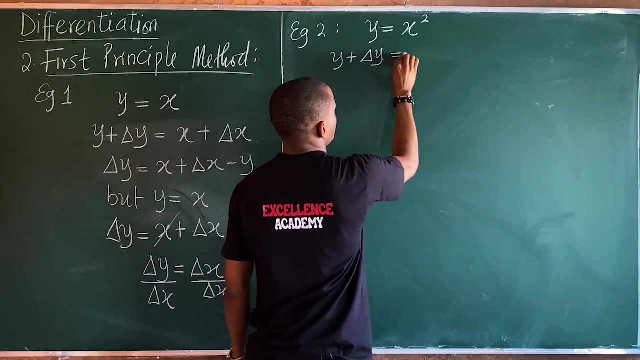 to what there? to x. but let's do this, man, using um first principle method. so what's the idea here? so we said, don't forget. we said from this, we said: to y, add change in y to x, add change in x, so use this concept. here becomes: i'm having y, so to y, i'll add change in y is equal to i'm seeing x. 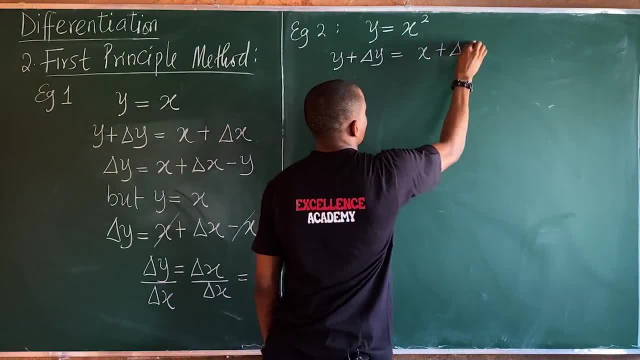 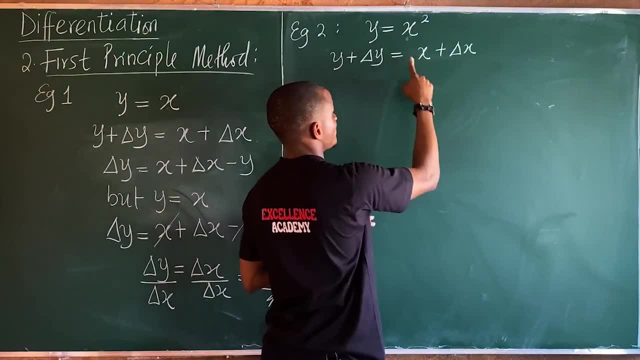 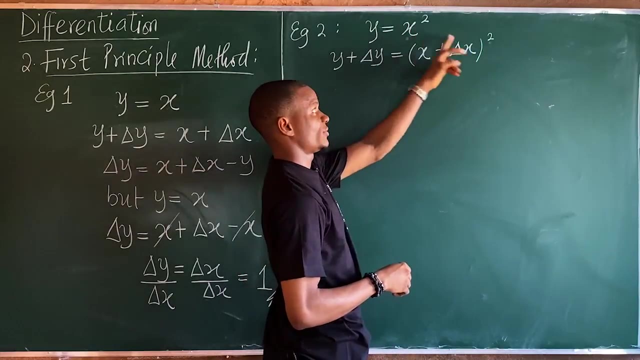 so becomes x plus what's there? change in x. but what do you notice? notice that, unlike in this case, here for this x the value is squared, so becomes x plus change in x. i will square this, reason being that my x value here was squared, so becomes this squared. all right, work on this. 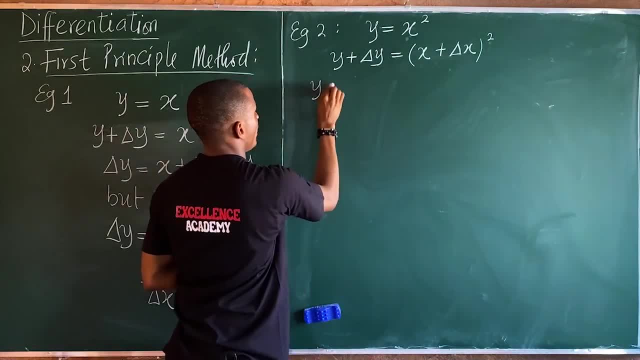 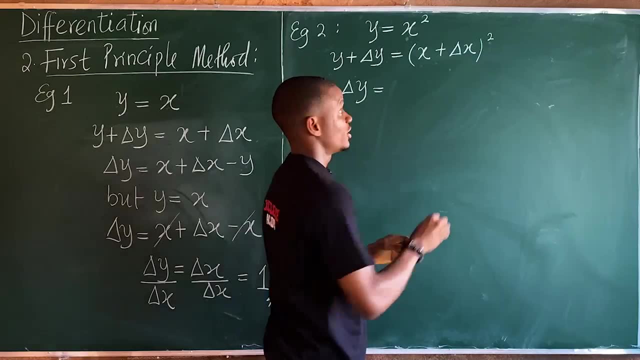 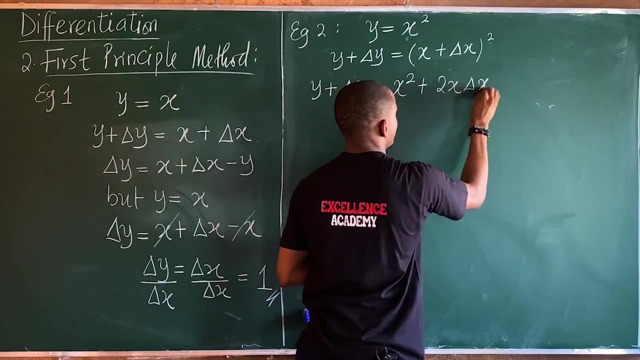 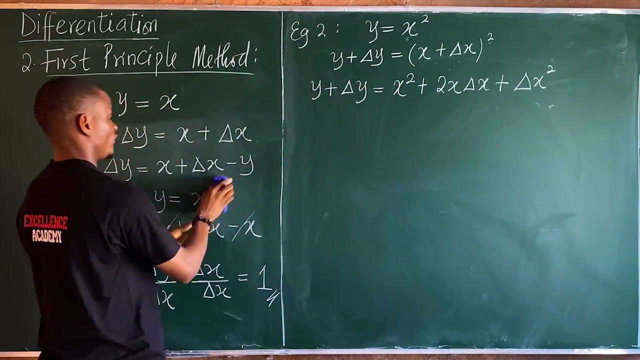 i'll have to expand this. i have that y plus change in y is now equal to. if i expand this using binomial expansion, this will give you x squared plus 2x, dx plus. this gives you the x squared. that's using the concept of binomial expansion or perhaps pascal's triangle to do this expansion. 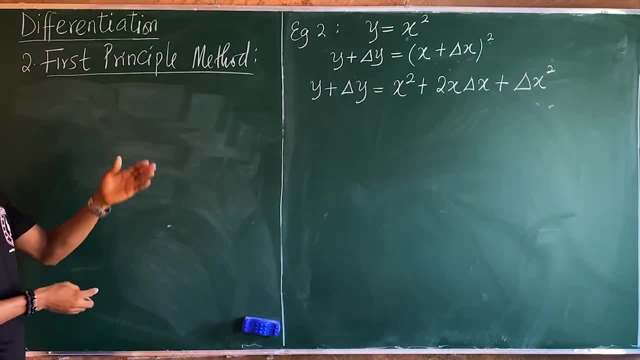 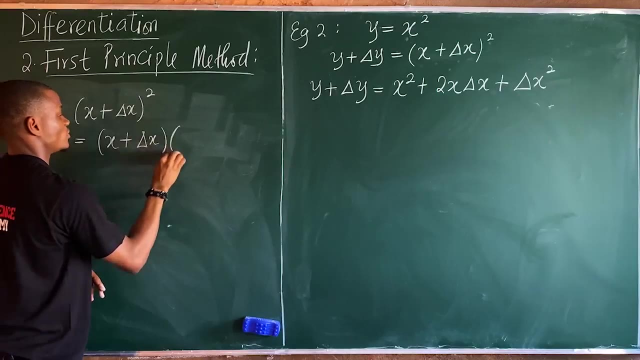 but for the sake of teaching, let me expand this separately. so i'm seeing here as x plus change in x, all squared. once something is squared, it means it is multiplying itself. so it now becomes x plus change in x, multiplying x plus changing x. this is this squared multiplying itself. 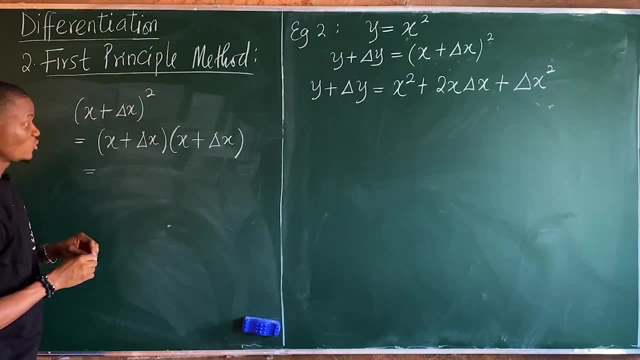 this is now equal to. so the concept here is to use each of the terms in the first bracket to multiply all the terms in the second bracket. use each of the terms in the first bracket to multiply all the terms in the second bracket. so i'll take this first term here: x, multiply everything here, x plus change in x. take the. 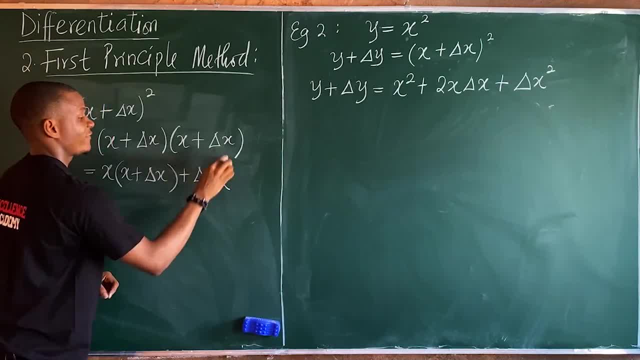 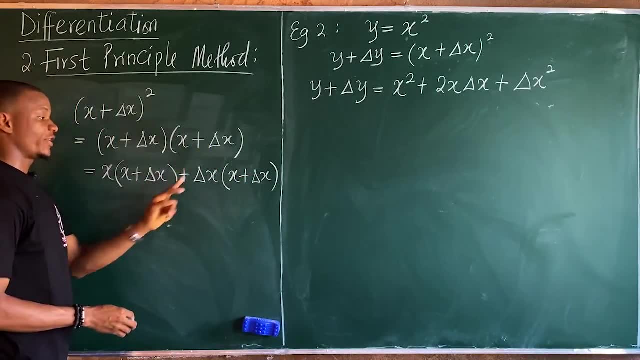 second term here, plus change in x. multiply everything here: x plus change in x. so take each of the terms in the first bracket, multiply everything in the second bracket. this is now equal to x times x gives you x squared plus x times changing x gives you. please, mind you, it will not. 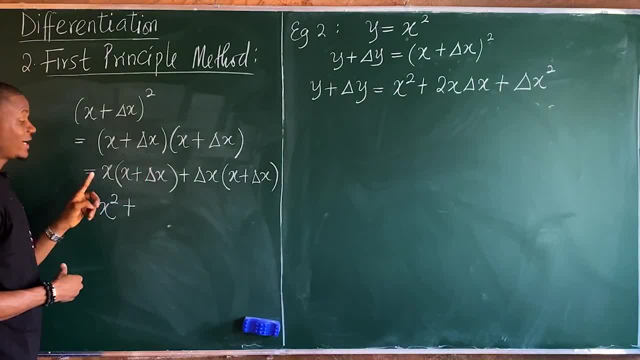 give you change in x squared. no, we're assuming that x and changing x are two different things. so you can see x times changing x equal to changing x squared. that will be wrong. it becomes x changing x instead. so x times changing s gives you x changing x and not changing x squared. 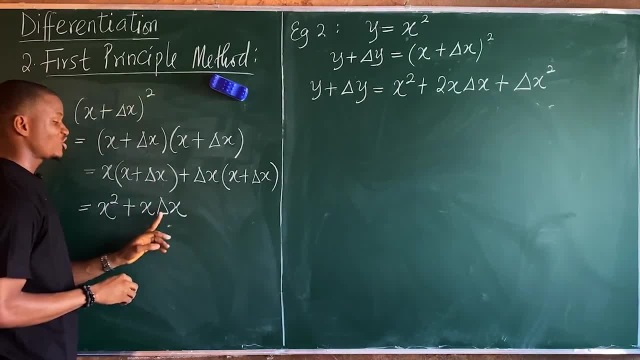 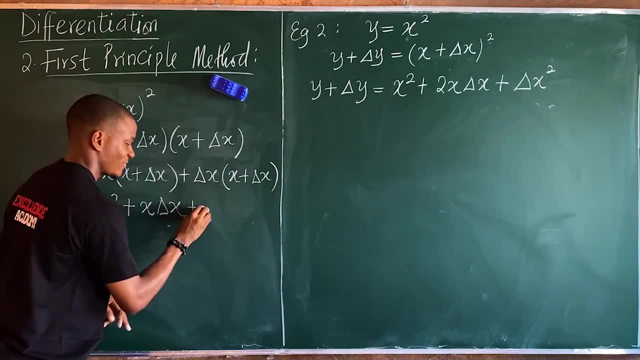 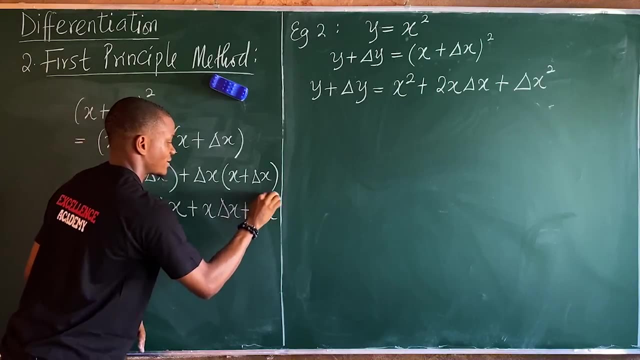 this will be wrong, please. so i'm having x times changing x is x changing x plus same concepts here: changing x times x gives you the same thing, x changing x. so i'm having x changing x plus changing x times. changing x gives you changing x squared. if i work on this now, it's equal to 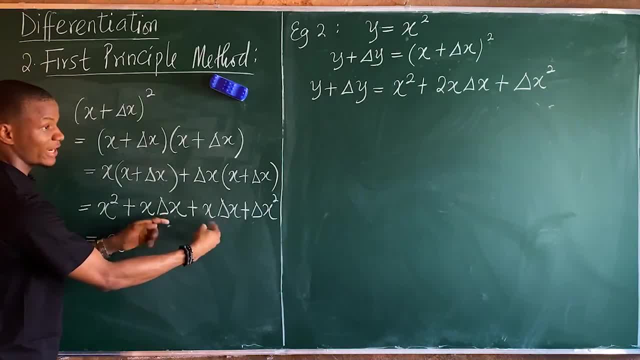 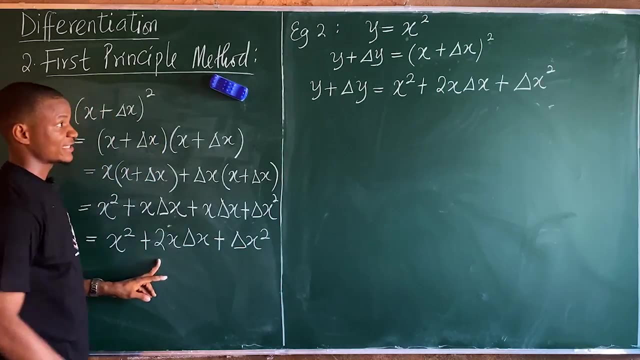 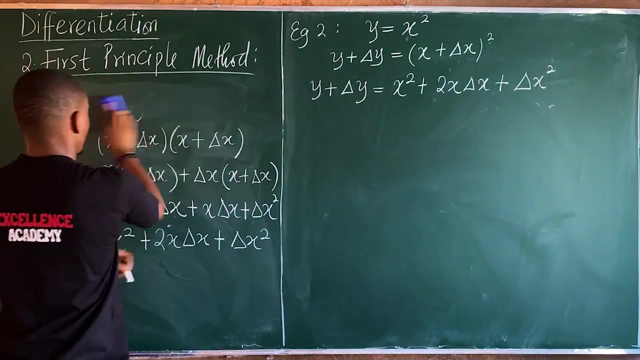 i'm having x squared. these two are like terms so they can add up. so x changing x plus x changing s gives you two of it becomes plus 2x changing x plus finally changing x squared. and this is how i arrived at this answer. all right. next up, if you refer to the previous example, we said: 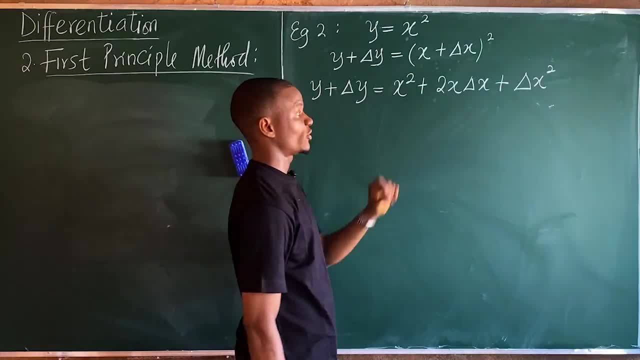 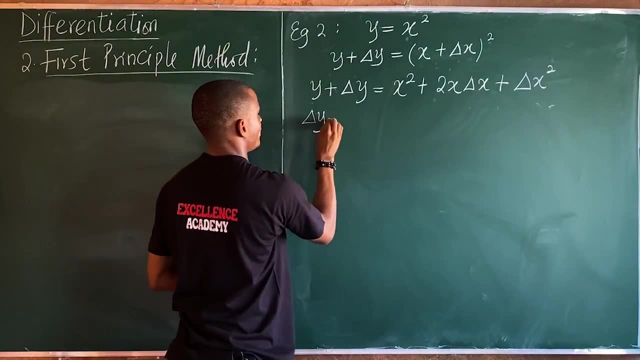 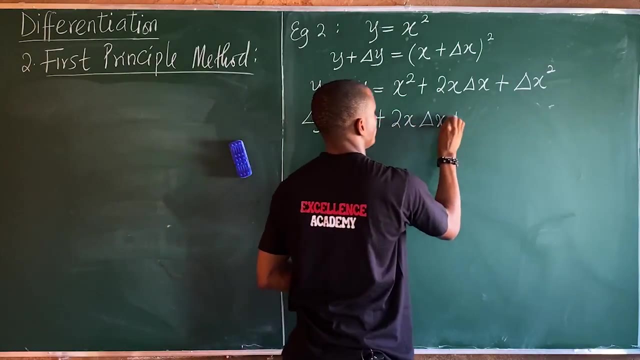 at this point, after your expansion, i'm done with my expansion here. after this: now i'll move the value of y over here, such that i'll be this: now i'll move the value of y over here, such that i'll be that changing y is equal to this, is x squared plus 2x. changing x plus changing x squared, i'm. 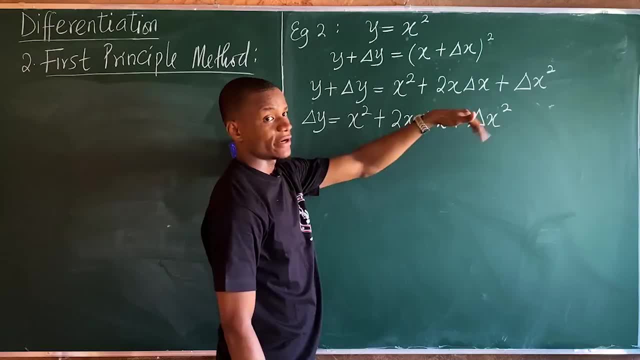 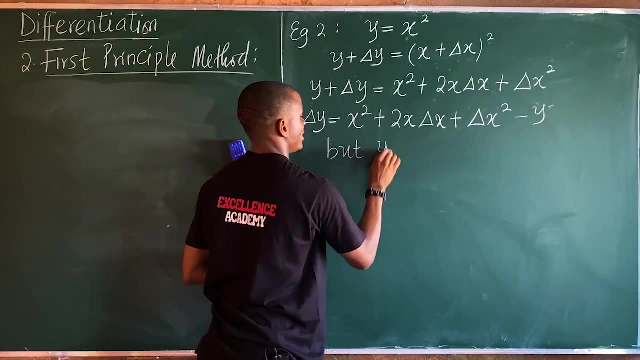 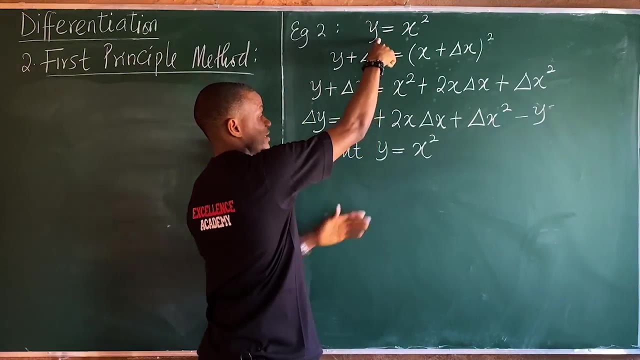 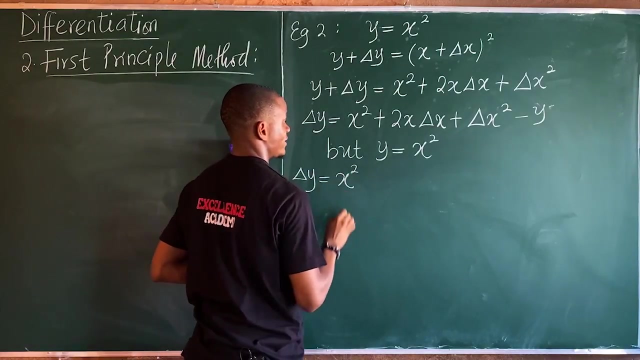 having a plus y here moves over. here becomes what? now minus y? so it becomes minus y. but i already have a value for y. but we said y is equal to what. x squared becomes equal to x squared. from here, y is equal to x squared. hence i will have that changing. y is equal to x squared, plus i'm having. 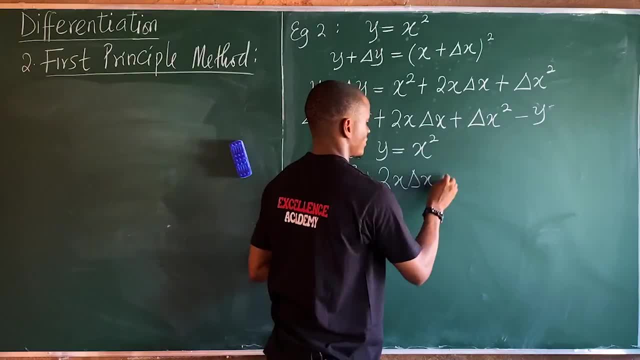 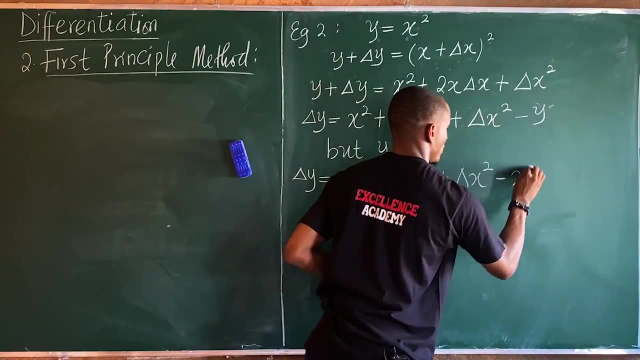 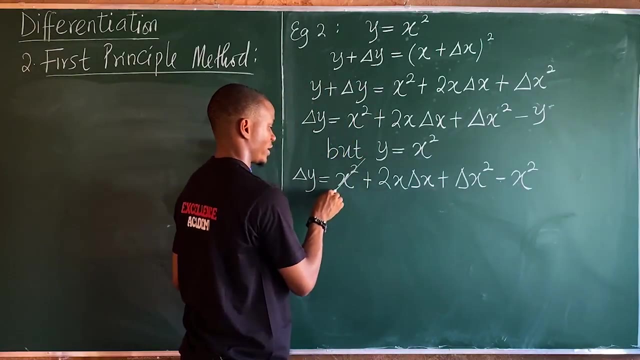 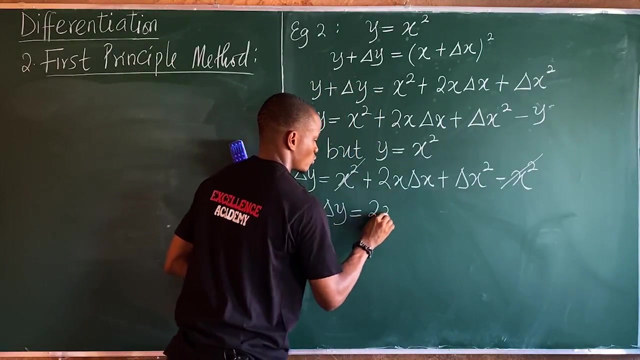 this as 2x changing x plus changing x squared, minus y. what's y there? x squared, so becomes minus x squared from here. i'm seeing x squared, i'm seeing minus x squared, so this one here would cancel this and i'm left with change in y being equal to 2x changing x plus changing x squared at this point. 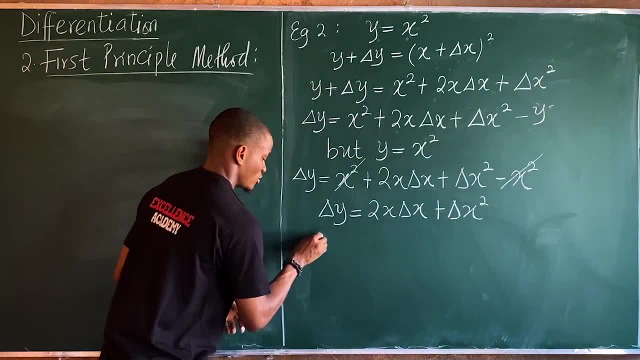 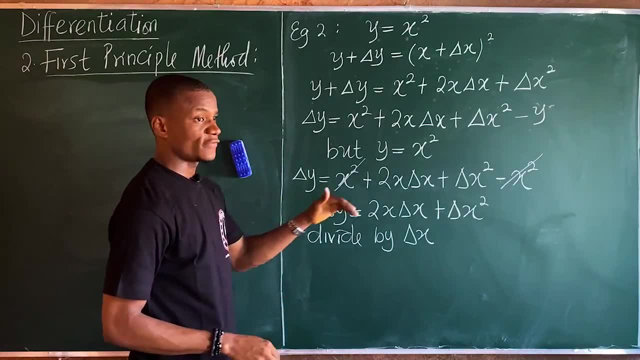 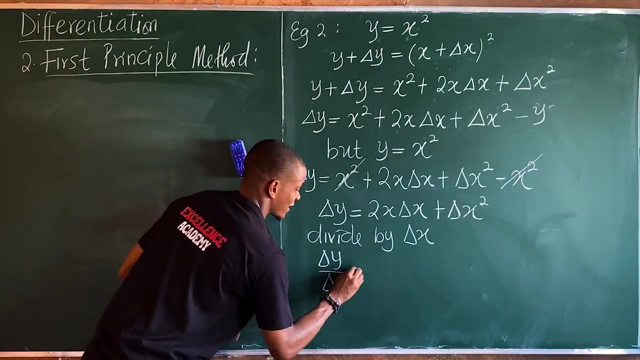 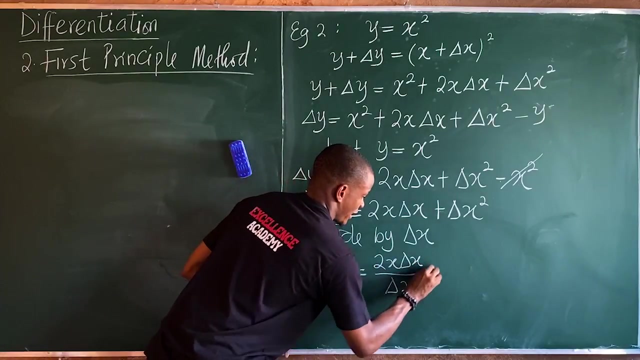 now i'll divide through by changing x. so if i divide by changing x, i'm mind you i'm dividing each of the terms by changing x, so it becomes change in y all over. changing x is now equal to here becomes 2x. changing x all over, changing x plus. i'm having here as changing x squared all over. 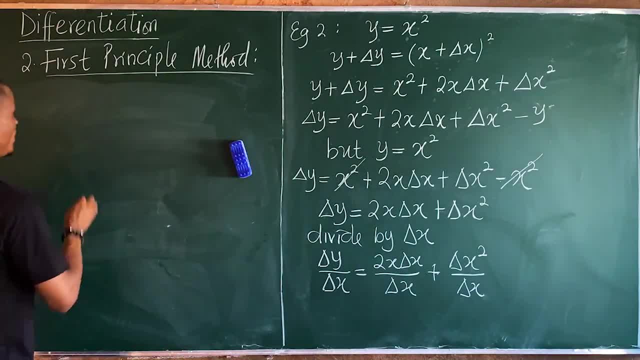 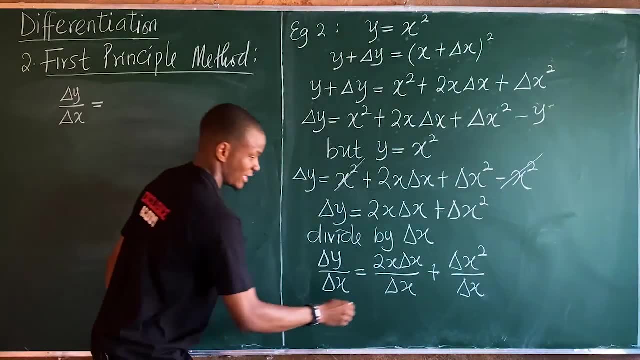 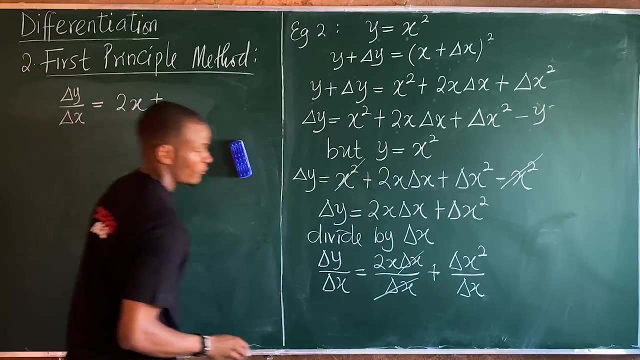 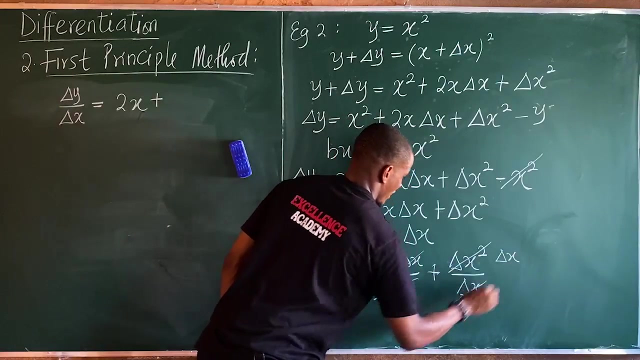 changing x. right, if i work on this now, i'll have that change in y all over. changing x is now equal to: from here now. this cancels this. i'm left with 2x becomes 2x plus from here now. this is of it. that's why it's squared. this cancels this. i'm still left with changing x, so it becomes. 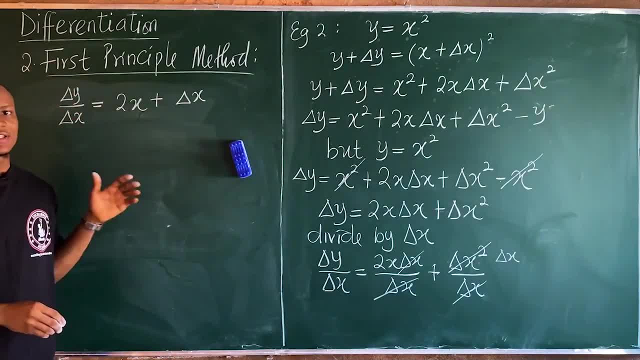 plus changing x. notice the difference between this example and the first one. for the first one, after doing this, i had just x there. oh, so i had just one there. in this case, now, after getting your change in y over changing x, if you still have a change in x here, what do you do now? i'll take limits.